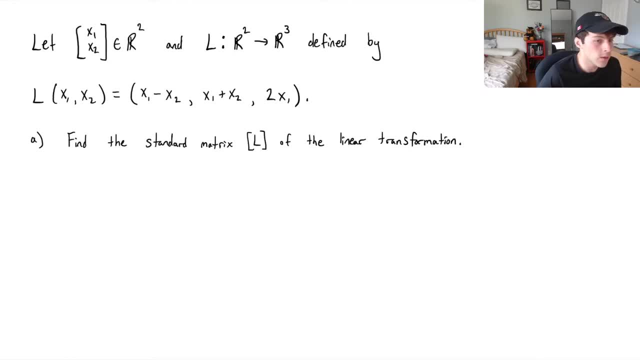 And it goes from the domain of R2, transforms it into a vector in the vector space R3, which is our co-domain, And it's defined for us in this way here, where each of the components of our vector in R3 is just made up of some sort of addition, subtraction or scalar multiplication. 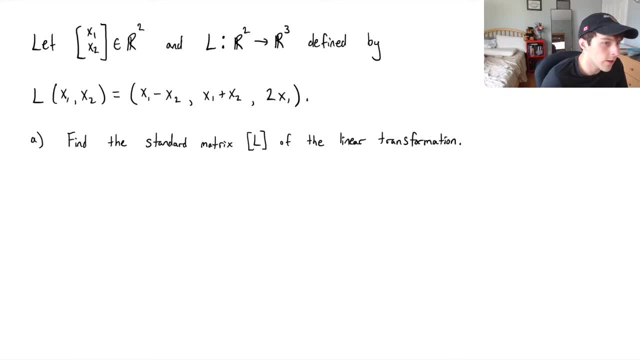 of the vector space And then we're given the individual components of the vector. that goes into our domain. So find the standard matrix L of the linear transformation. So finding the standard matrix that describes this linear transformation, if the linear transformation's already been defined for you. 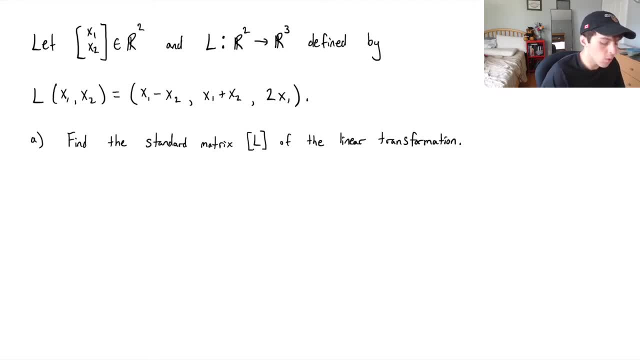 this makes our life a whole lot easier, because all we need to do for this is to plug in the standard basis vectors of the domain into our linear transformation, and this will make up the columns of our standard matrix. So let's begin by doing that. 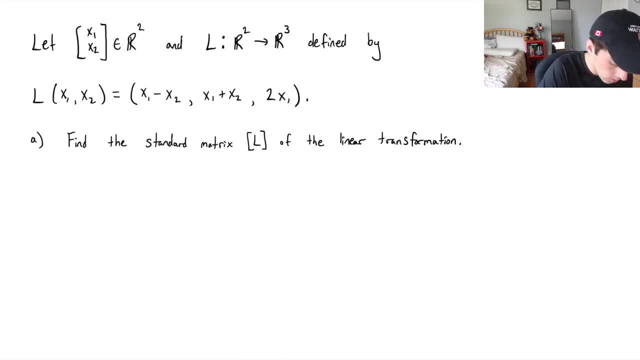 So, starting with the linear transformation of- and remember, the standard basis is given by these elementary vector, lowercase e sub 1.. And I'm also just going to write this out for clarity. I'll write this in this way. I'll write this in the vector form as well, but e1 would be the exact same thing. 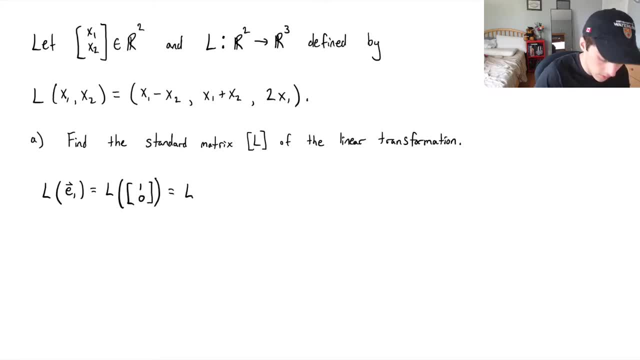 So you might also see this as 1, 0, like this. These all are meaning the same thing. they're just different notation And since it's defined, we know that the first element is 1 minus 0,, the second element is 1 plus 0, and the last element will be 2 times 1.. 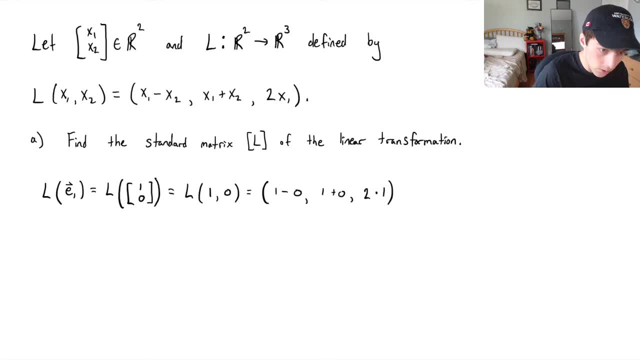 So this is going to give us the vector in our 3, 1, 1, 2, right And I've written it in that form that it's given us, but if you prefer this square bracket notation, writing it like the transpose. 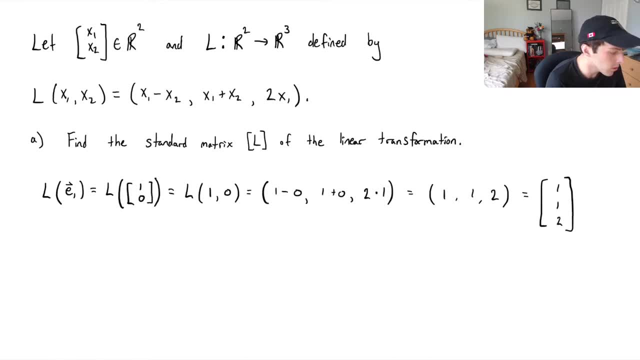 nothing wrong with this. If this makes more sense, I would just go with this. So this is what the first standard basis vector of the domain is, The first standard basis vector of the domain maps to of this linear transformation. Let's do the exact same thing now with the second standard basis vector. 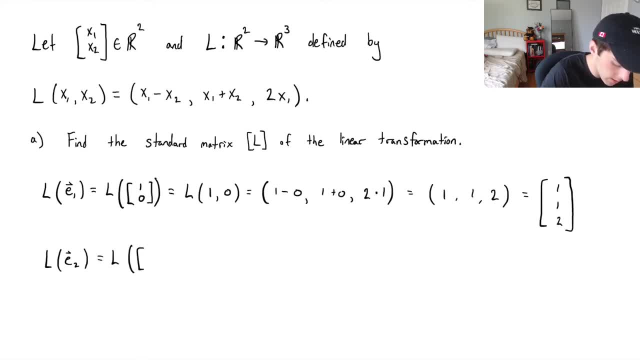 And this is like 0, 1.. This is going to be 0, minus 1.. This is going to be 0, plus 1.. And it's going to be 2 times 0.. So, lastly, we are going to get negative 1, 1, and 0. 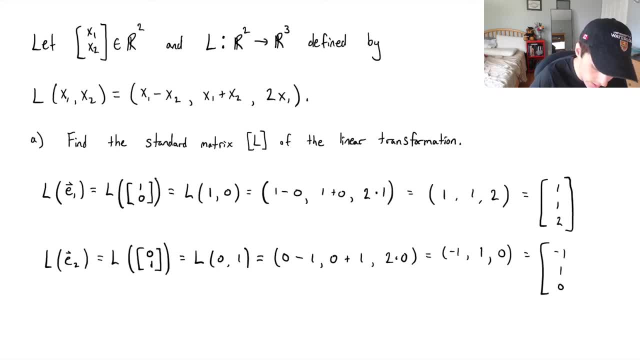 Or negative: 1, 1, 0,. written this way: Same thing. I've clearly written out a lot of different notations here, but in general you just stick to the one that you want. And yeah, I mean, typically, if you're comfortable with all of them, you're going to be fine. 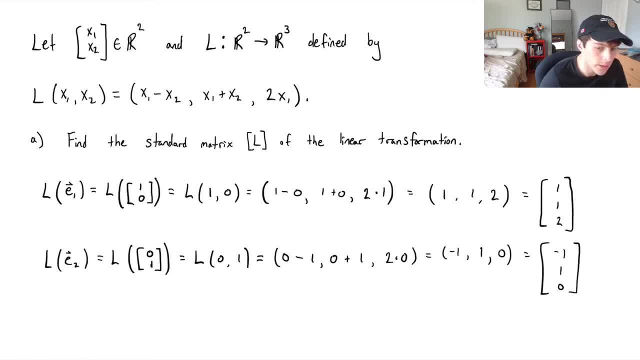 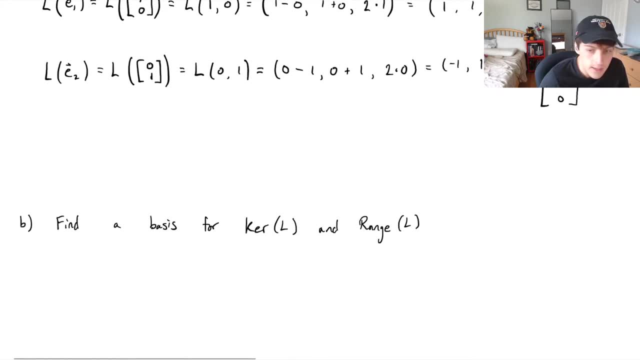 But typically, if you're comfortable with all of them, stick to the same notation that's given in the question. Okay, And let's scroll down here. Okay, And remember the standard matrix that describes our linear transformation. well, the first column is just going to be L of E1.. 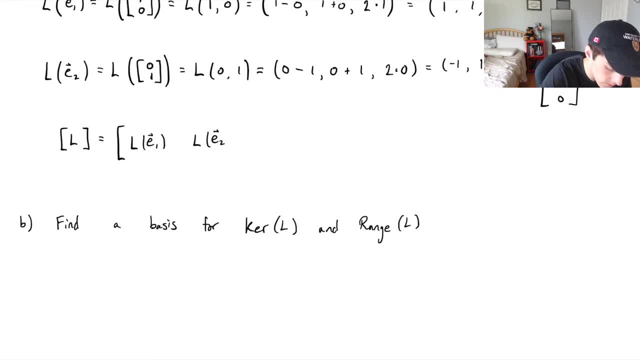 Second column will be L of E2.. So we know that this will be 1, 1, 2.. And our second column will be negative: 1, 1, 0.. Okay, So this is the matrix that describes our linear transformation. 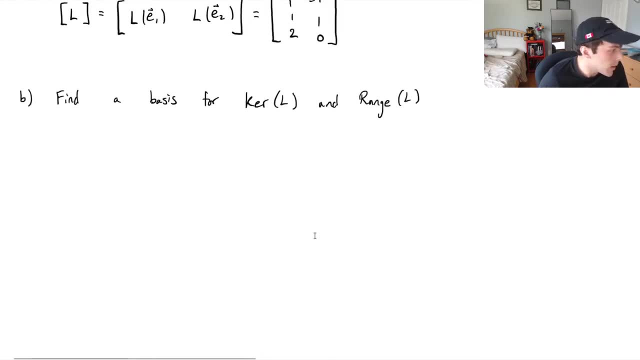 So next, this is asking us to find a basis for the kernel of L and the range of L. So let's do a little bit of a refresher of what these actually mean. Well, we know that the kernel of L is just going to be, it's all. 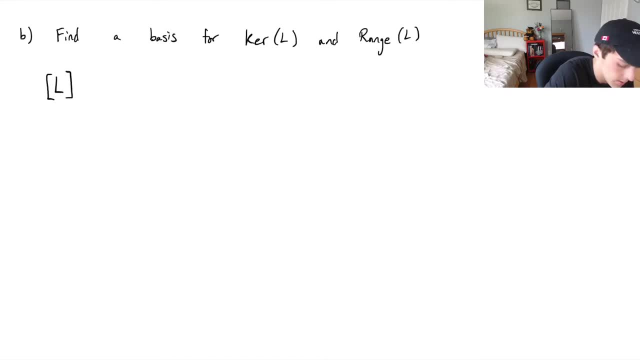 remember, our linear transformation can be expressed as this standard matrix L times a vector x, And when this is equal to the zero vector, well, the kernel is going to be all of the vectors x. that, when multiplied by our standard matrix L. 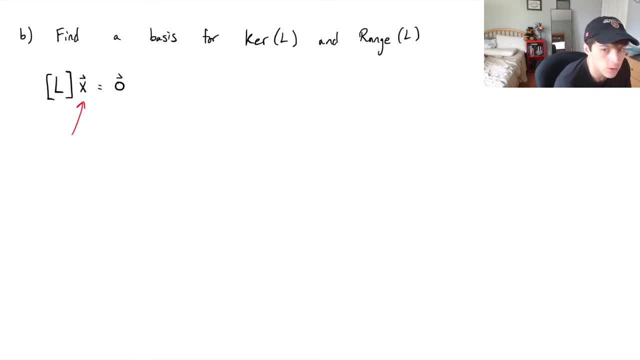 will map to the zero vector of our codomain Right. So another way that you might see this written in like a textbook is like: if we take the linear transformation of a vector x and it's equal to the zero vector right. 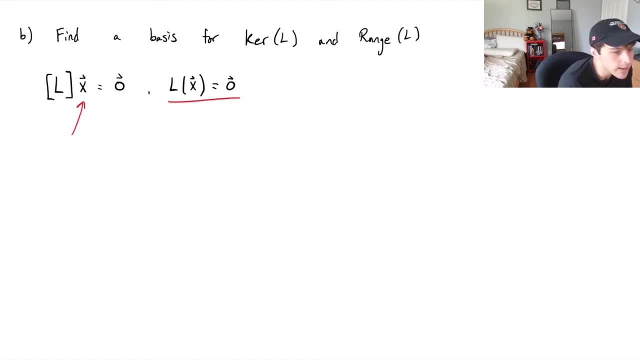 you probably see it just described like this And it's the exact same thing. It's just when I first wrote it. I wrote it in terms of this matrix vector product of our standard matrix L times a. vector x is equal to the zero vector in R3.. 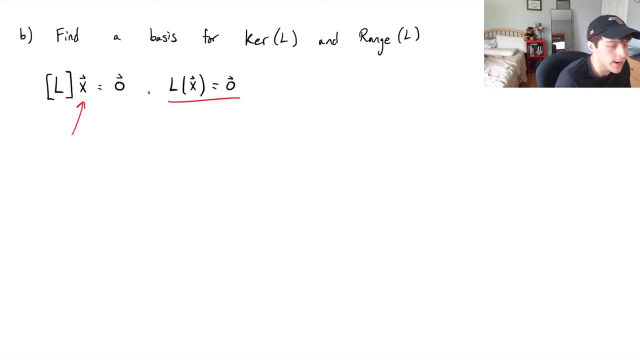 Except you can see it's a lot neater when you just write it, as linear transformation of x is equal to zero, Right? So same thing. But you'll notice that this is like, by definition, the null space. If we had like: ax equals zero, right. 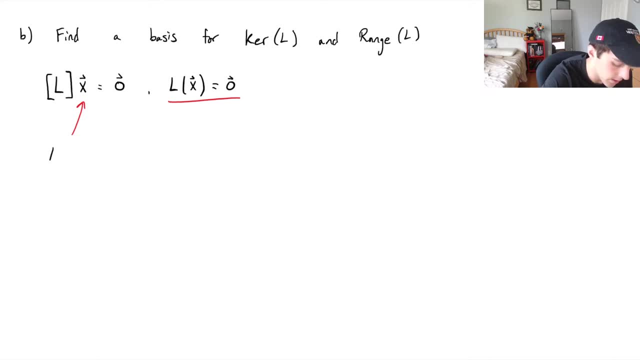 some matrix vector, product ax equals zero. well, all of the vectors x that satisfy that equation will be the null space, Right? So you can see how these are very, very related concepts. And we can see how, if this is just the null space. 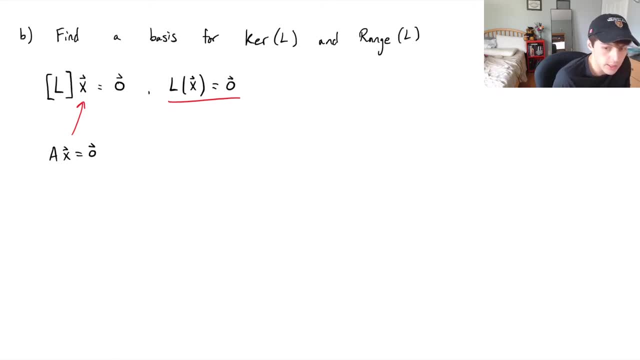 then we should solve it pretty much the same way. We just need to set up a matrix of our homogenous system. L times x equals zero vector row. reduce this and then we'll interpret the results from there. So let's set up a matrix. 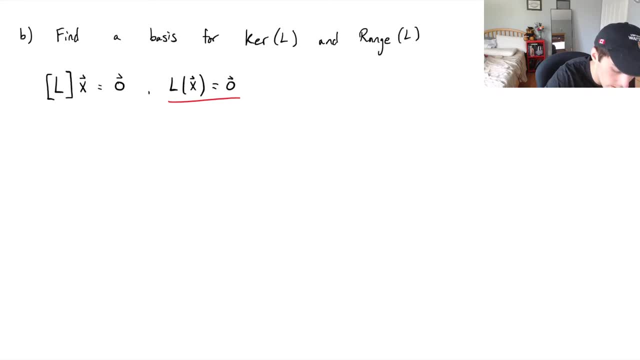 Right. So we know we already did our, or found what our matrix was, our standard matrix It was this 3 by 2 matrix, right here. So now let's row reduce this, And I'll go through this somewhat quickly. 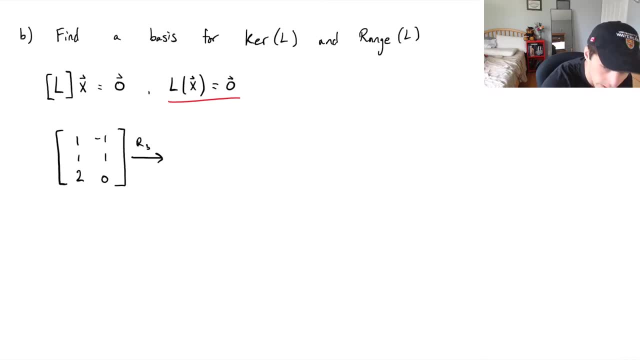 So let's do: r3 is going to be equal to r3 minus 2 times row 2.. So this will be zero, This will be minus 2.. This will stay the same And then we can do: row 2 is going to be equal to. 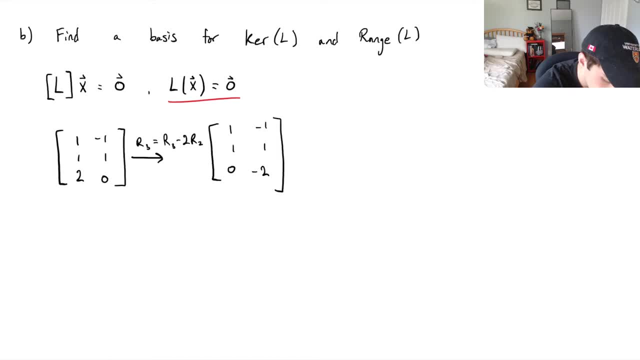 row 2 minus row 1.. Just trying to get rid of the non-zero entries underneath the top left entry of this matrix, Alright, Next, we're going to try to get rid of that bottom right entry, So we can do. row 3 would be equal to. 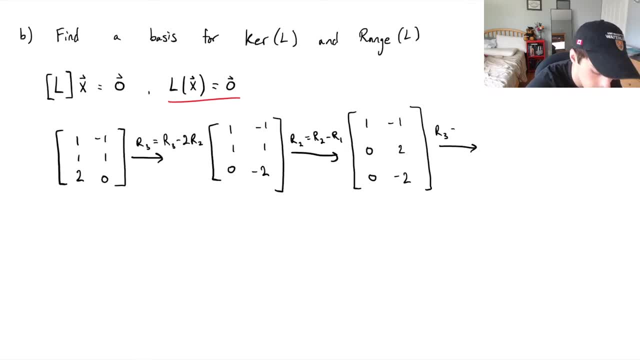 row 3, and we're going to add row 2 to it. And then, lastly, let's just divide. We'll divide row 2 by 2. And we'll be left with 1, 0, 0.. 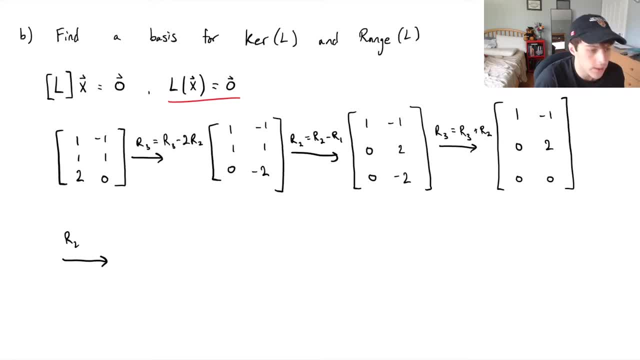 Negative: 1, 1, 0.. And we can see now that we are in row echelon form And from the row echelon form, well, we can see that, since there's no free variables here, or the rank of this matrix is equal to the number of columns that we have, 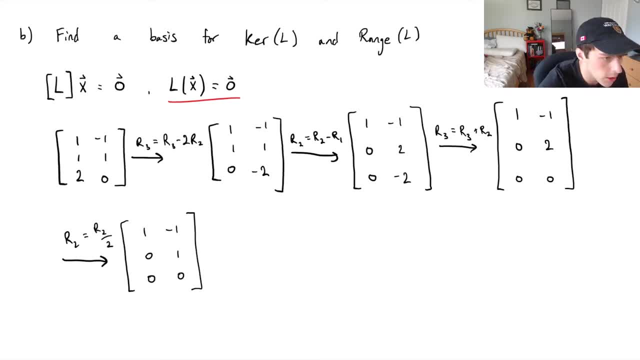 well, we can see that the only solutions to our homogenous system would be the zero vector. And if that's not entirely clear, then let's look here. Remember this first column: if we're solving this matrix vector, product L times. 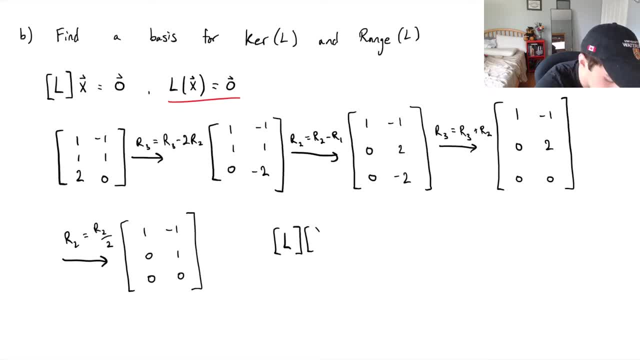 let's write this as x1, x2.. This is equal to 0, 0, 0.. Then the solutions to this system. remember, we're solving for this x vector, right, And you can see here right. 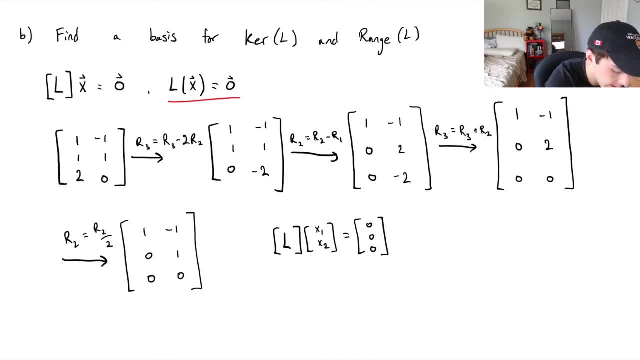 this first column and this second column of our row echelon form, we can see that those represent the components x1 and x2 of the solutions that we're solving for Right, All of the vectors x that satisfy this homogenous system, this matrix vector product. 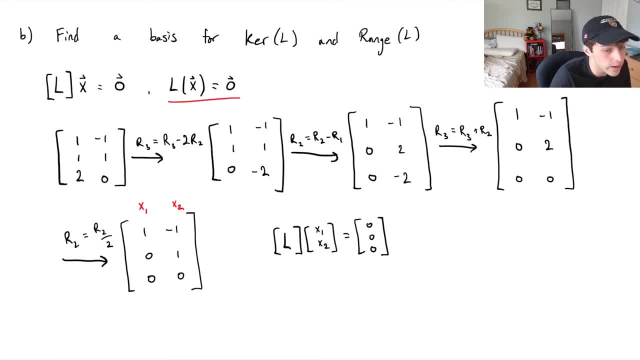 Right, So we can see that since there's no free variables x1 and x2, they have to be equal to 0.. Right, The zero vector is the only solution to this matrix vector product. Right, So if x equals the zero vector, 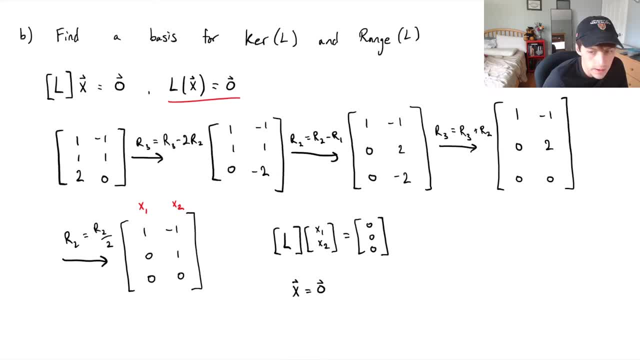 is the only solution, then that means that the kernel of the linear transformation only consists of the zero vector Right. So we can write this as well: the kernel of L is equal to- and remember, this is a set of vectors. 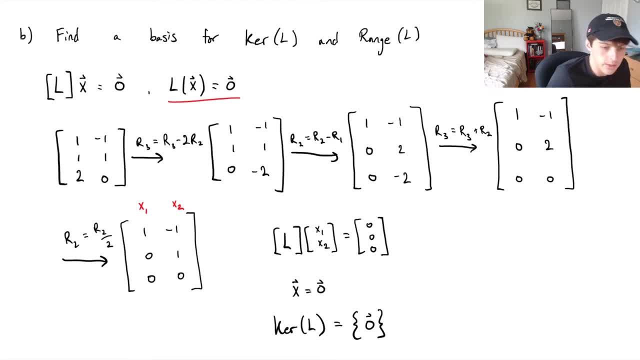 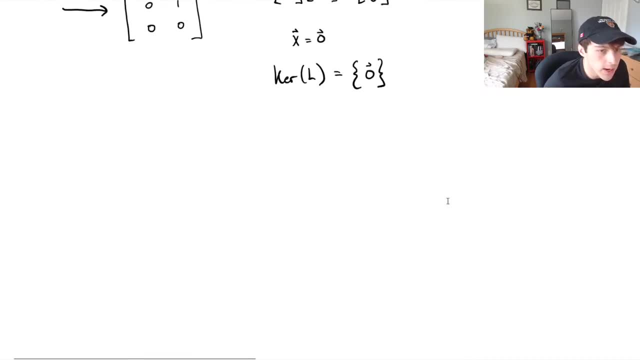 but it's equal to the set of vectors, which only contains the zero vector. And if you're asked about the basis of the kernel, it's not asking you for the kernel, it's asking you for the basis. Well, careful here. you know that if a set of vectors 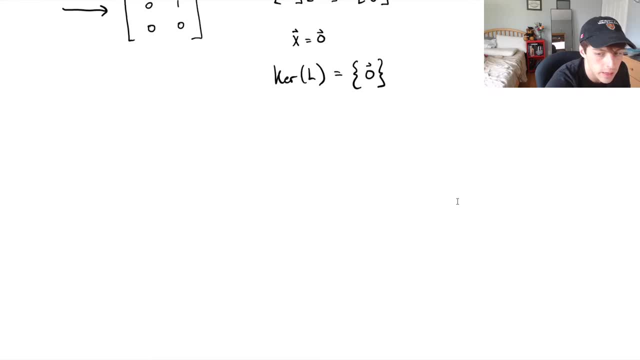 only consists of the zero vector, then it follows that the basis of that set of vectors would be the empty set, which is basically just the set of nothing, And it's a little bit confusing. I probably can't explain it, as well as some other sources that you might find online. 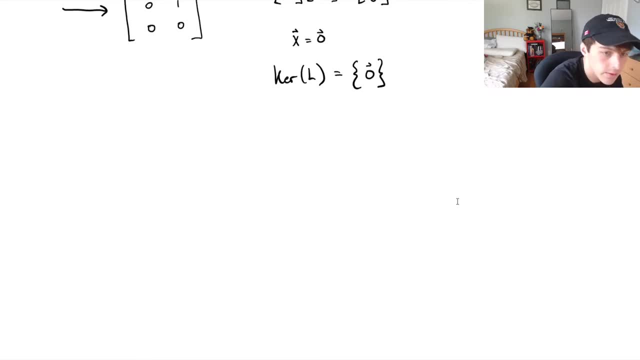 So just remember that the set of the zero vector, the basis for that set, is the empty set, And you can denote that as just this symbol right here, like this. So we can say thus: the basis for the kernel of L. 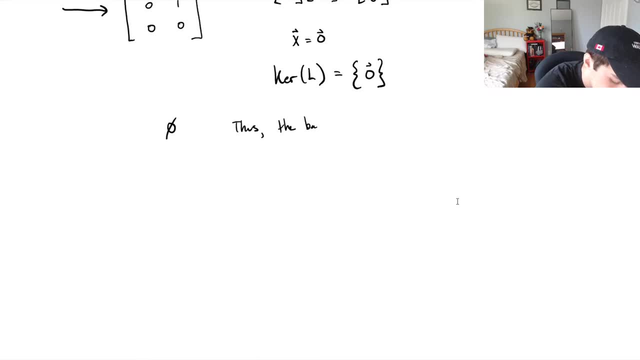 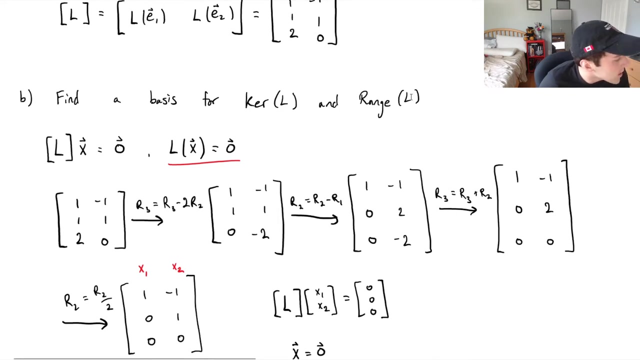 is the empty set. and here we are. Sorry if this video is a little choppy. my internet connection is being kind of dodgy. So we've answered the first part of the question right, But we're also asked about the range of L. 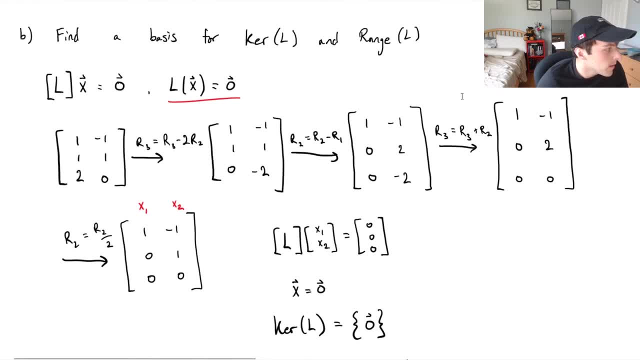 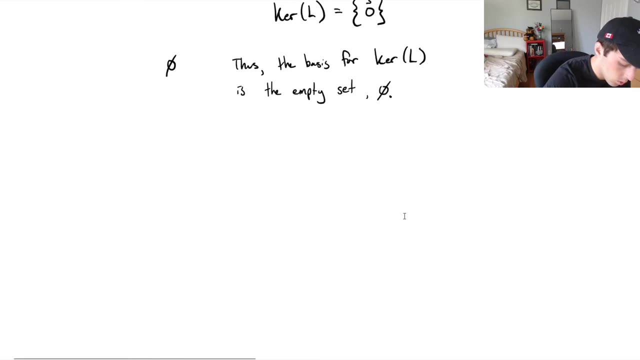 and the basis for the range of L. And we were talking earlier about how kernel and range are very hand-in-hand with the null space and the column space of a matrix. So the range of L, Well, the range of L is just. 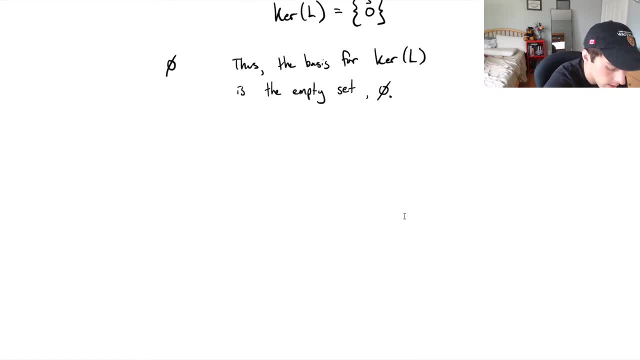 is all of the possible outputs of this linear transformation right. So L. it's like every single L right What this could be equal to. So if you plug in some vector x into this linear transformation it's going to spit out some vectors in R2.. 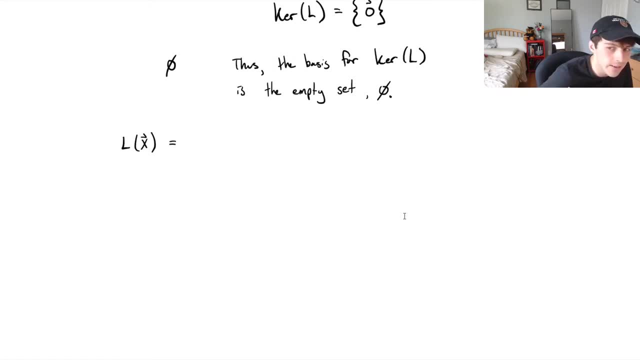 er R3, sorry. So the set of all of those possibilities is going to be the range of L Right, And you can see how that's super-duper similar to the column space Right. So if we had 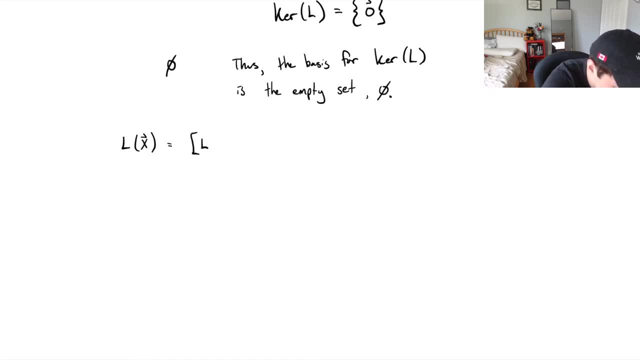 if we wrote this as standard, matrix L times some vector x, right? Let's write this a little bit differently: x1, x2.. Well, this'll just be. it'll be x1, by definition of matrix vector product right. 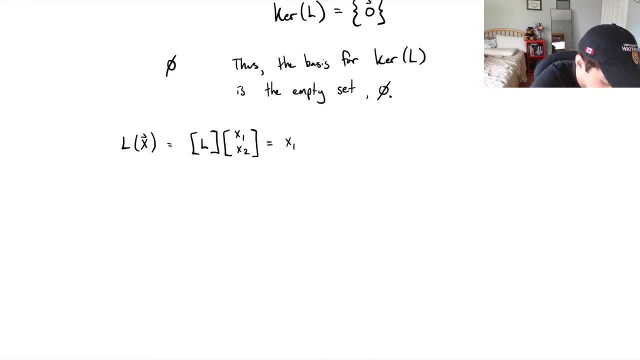 It's going to be the first column of L, which is going to be 1, 1, 2, er, yeah, 1, 1, 2.. Plus x2 times well, the second column of this. 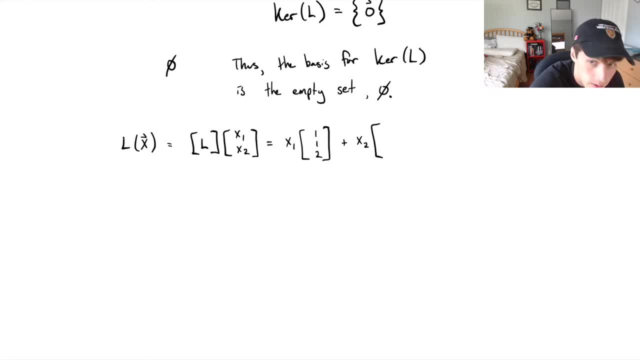 standard matrix L, we found was negative: 1, 1, 0.. Right, And this is for some x1, x2, which are just some scalars. right Because we're considering all possible x vectors, x in R2.. 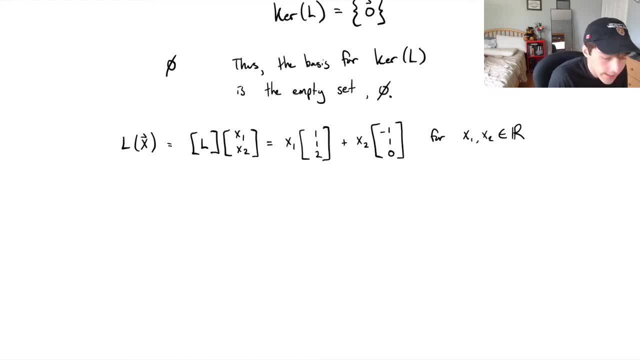 Right. So can you see here that if we replaced these x's with like scalars, like c1 and c2, you can see very clearly that this is the column space, right? This is the span of the columns. 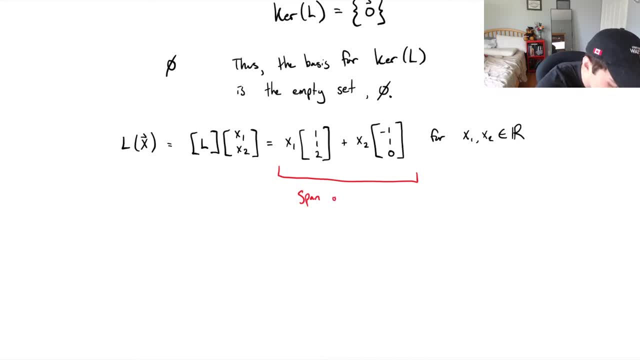 This is the span of the columns of L, Right. So you would solve it the exact same way that you would solve for the column space of some vector. So the range of a linear transformation L, you can see, is super similar to just the. 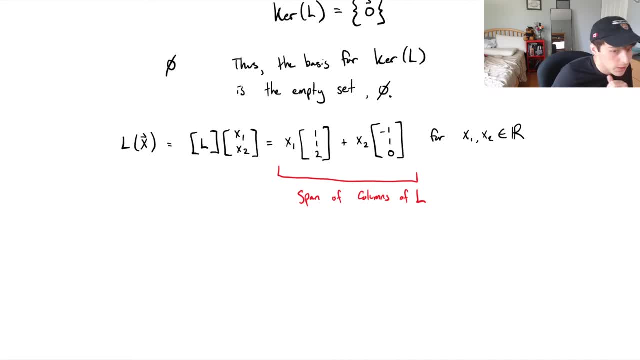 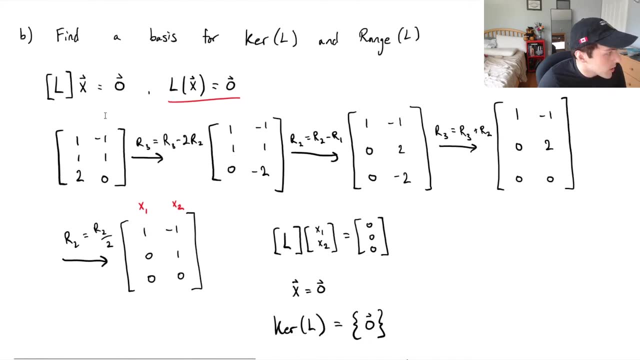 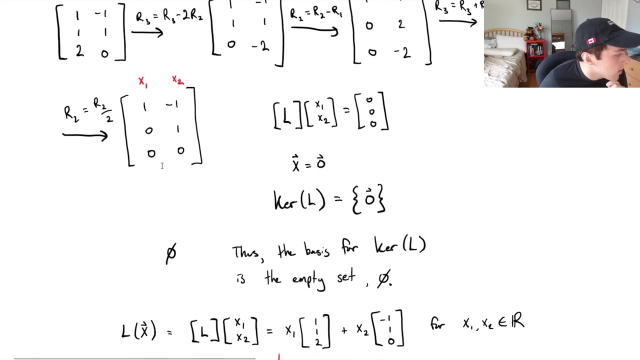 column space of that standard matrix L that describes the linear transformation. So since we've already solved this homogenous matrix or the homogenous system, right here we solve it the exact same way, Since we saw that x1 and x2. 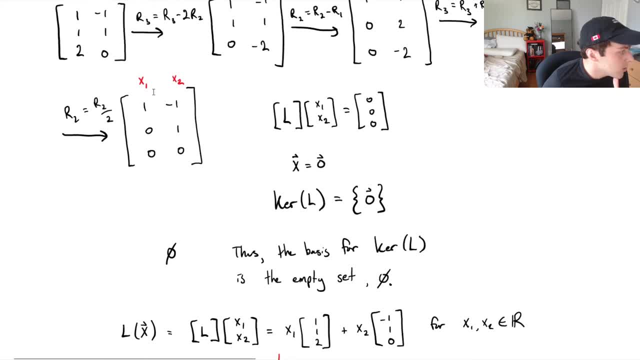 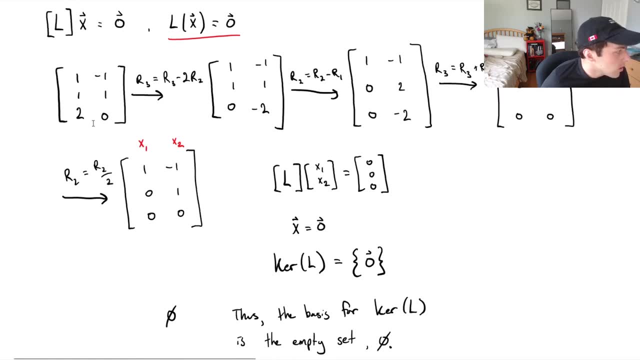 they have to be equal to 0, or there's no free variables. we know that the span is going to be just the columns of our standard matrix L. We have no free variables, so we can't remove any vectors from the span of the columns. 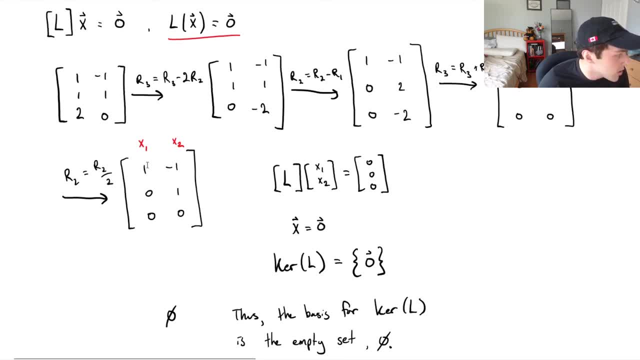 and have it span the same vector space. We can see that since there's no free variables, it means that the span of the columns we can't remove anything from there and they'll span the same thing. So it's simply just going to be. 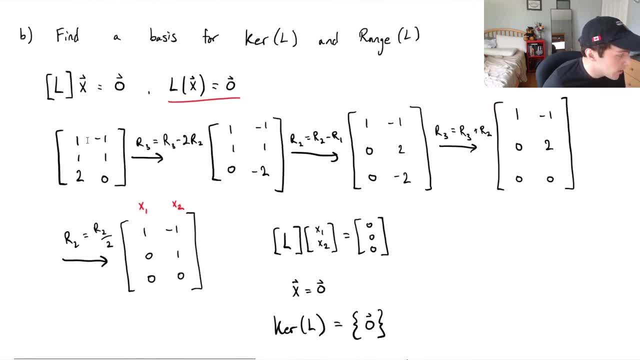 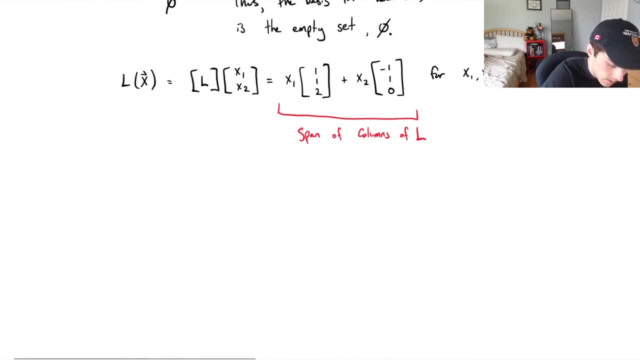 the span of the columns of our initial standard matrix. uh yeah, standard matrix L, So we can see. let me just write out in words what I just said. We see from from the reduced echelon- reduced echelon form of our 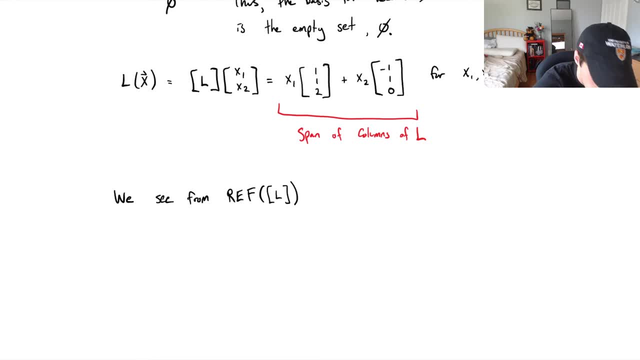 standard matrix L. we have a leading entry in column 1 and column 2. Thus we can say that the range of L is going to be equal to the span of column 1 and column 2.. And now, considering the basis of the range. well, 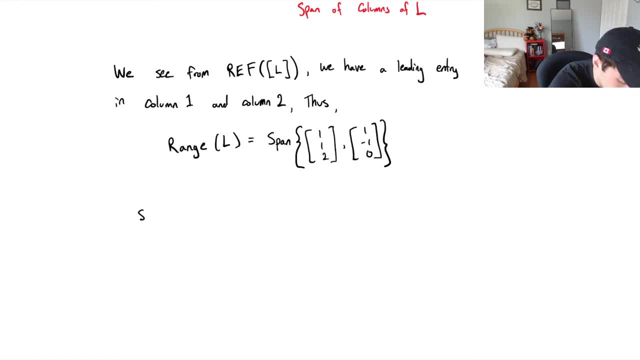 we can see that, since our vectors here 1, 1, and 2, and 1, negative, 1, 0, well, since that these are both non-zero vectors and they're both non-parallel, we can see very clearly that they're not. 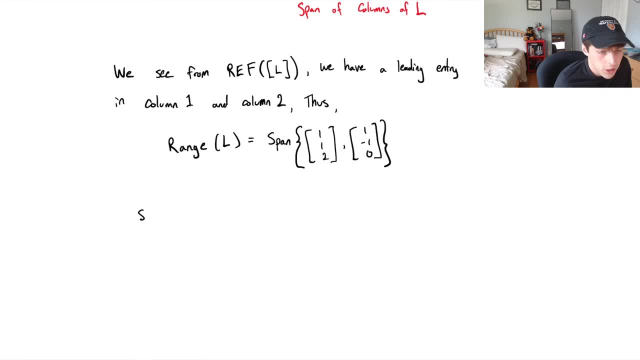 scalar multiples of each other, we can see that these vectors form a linearly independent set Right. And since they form a linearly independent set and they span the entire range of L, then that means that we can take the set of those two. 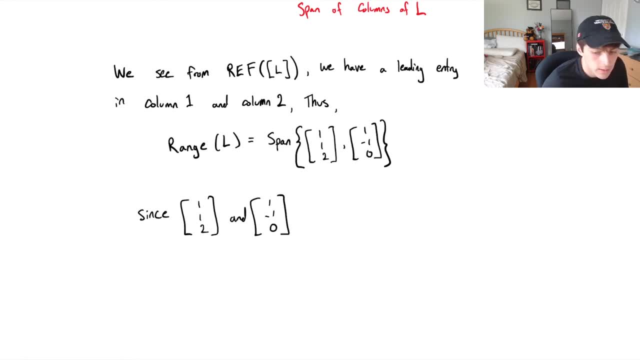 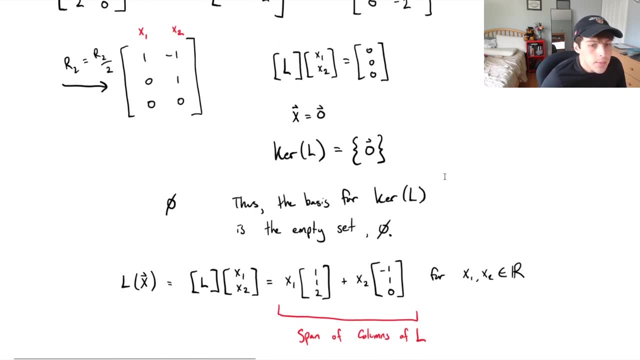 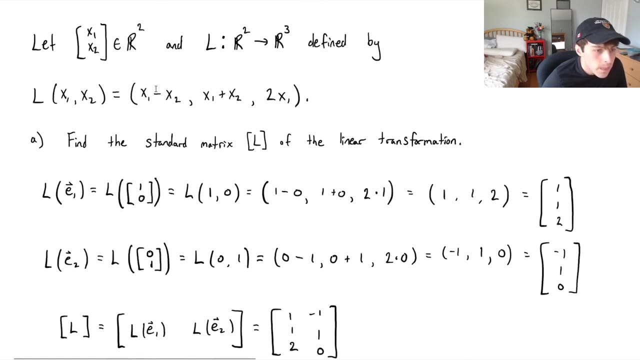 vectors and call that the basis for our range. So I've just written out exactly what we just said. So, to recap this video, we were starting off given a linear transformation and it was defined for us. We were then asked to find the standard matrix. 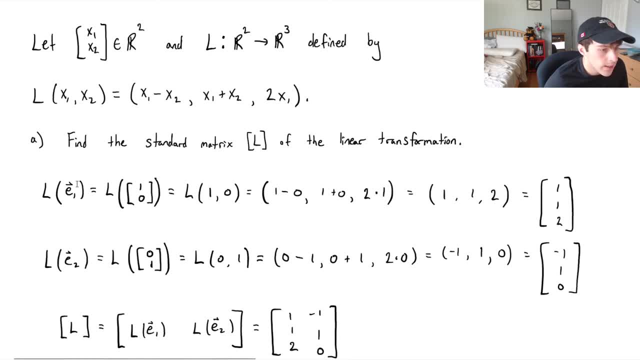 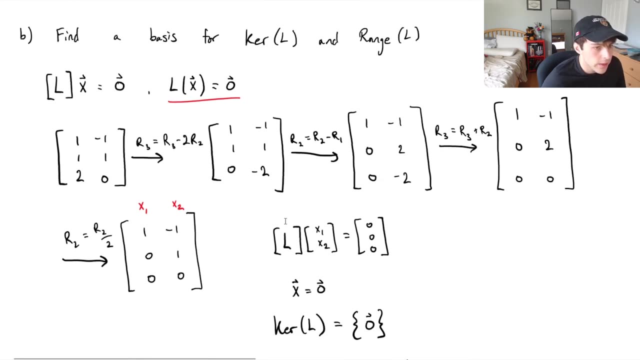 of the linear transformation. and we did that by plugging in the standard matrix vectors of the domain and finding out what those vectors map to. Those vectors become the columns of our standard matrix Once we found that we needed to find the basis for the kernel and the range. 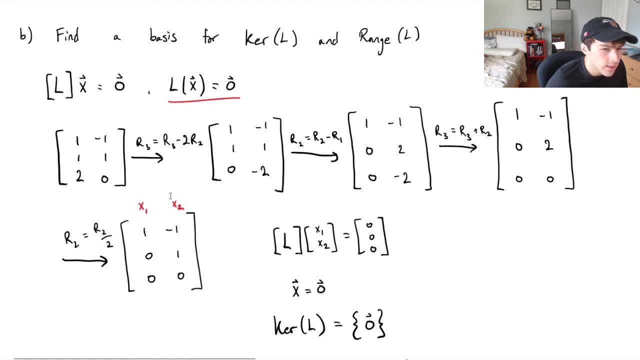 So we started off by finding the kernel and the range and then we interpreted our results to find the basis. The kernel was just all of the vectors that if you were to plug in to the linear transformation L, they would map to the 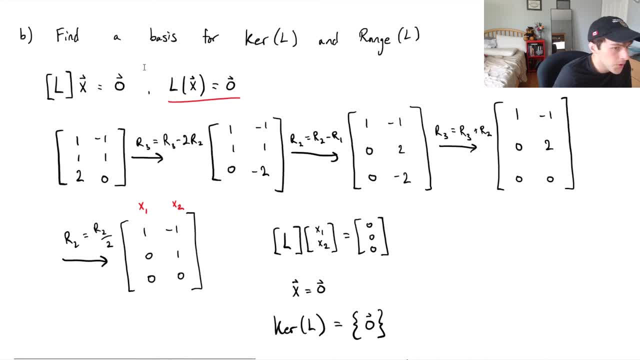 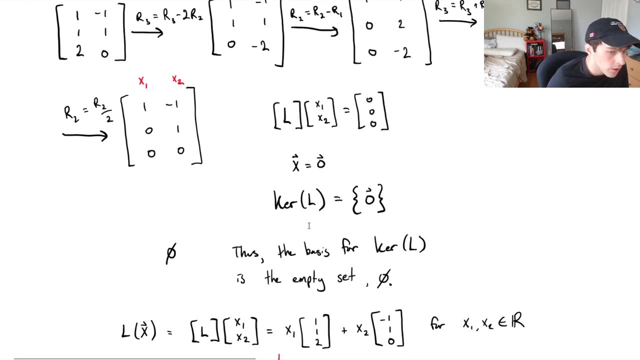 zero vector. We saw that this is very, very similar to the null space, and we solved our homogenous system and we found that the zero vector is the only vector that exists that maps to the origin of our codomain. Thus the basis for the kernel. 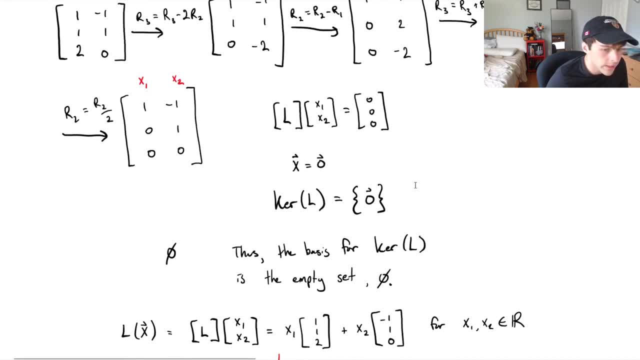 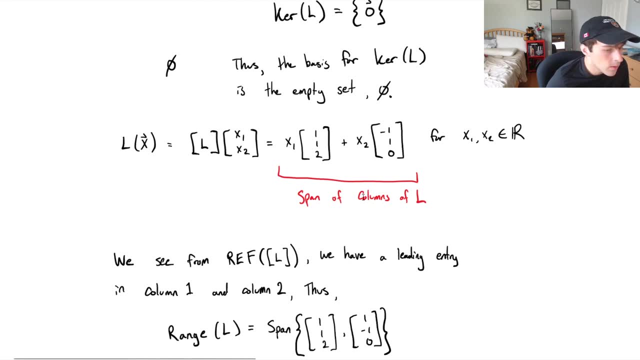 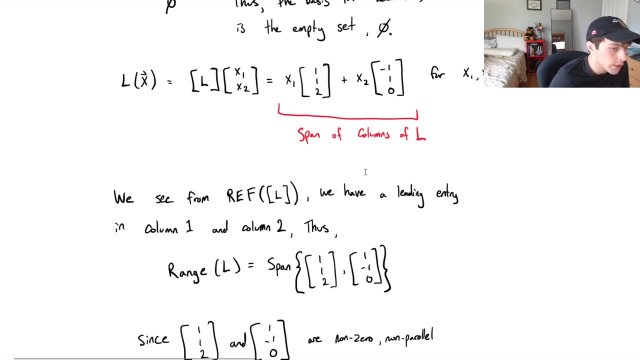 since the kernel only exists of that one zero vector, then the basis for this set will have to be the empty set. We also saw that the range of L is very similar to the column space of the standard matrix L. We saw that, since we have a leading entry in both. 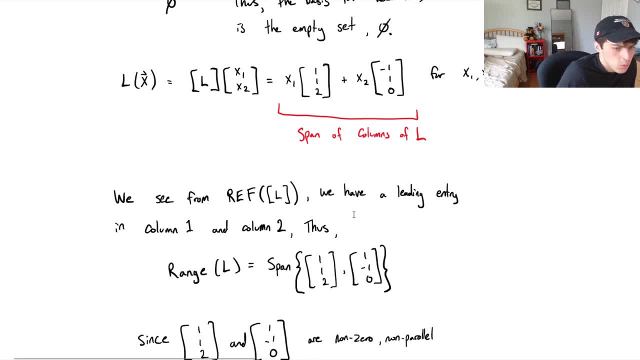 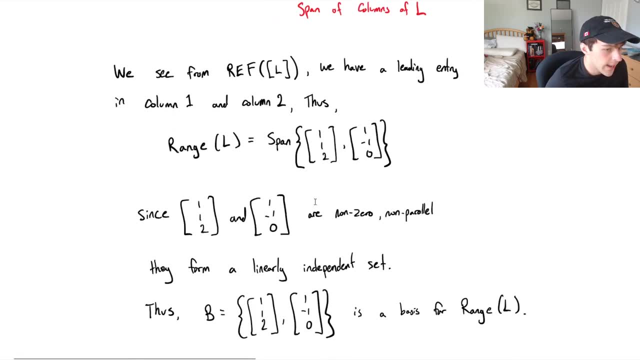 column 1 and column 2, and no free variables. we can take that the span of just the columns of our standard matrix L is going to be equal to the range of L, and it can't be simplified in any way. So 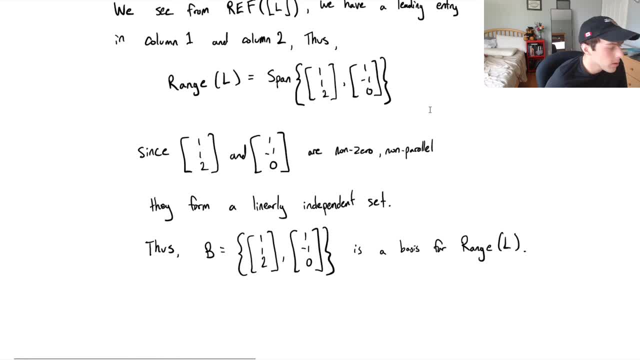 we noticed that since those vectors are non-zero and non-parallel, they'll form a linearly independent set, and since they span the entire vector space, which is the range of L, then we can call the set of those two vectors the basis.